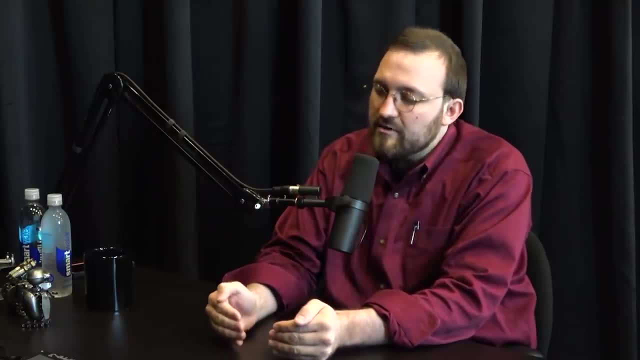 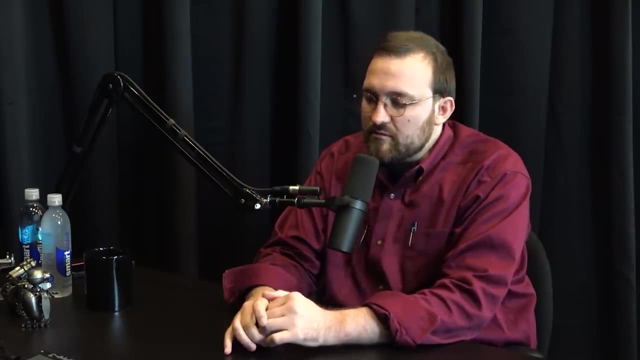 having a dialogue with a computer and thinking about: well, how would I solve that, How would I interact with that? What does this need to look like? Functional programming is what we've chosen to use for Cardano, mostly because we're living in the academic world. We've 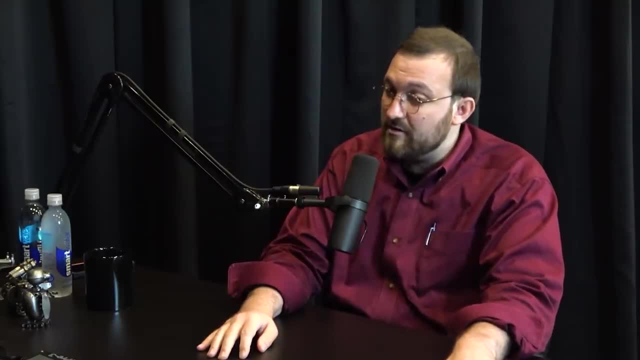 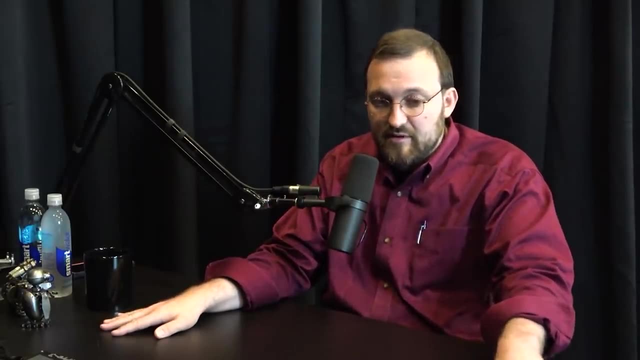 written 105 papers, And the problem is you have to translate that work into code, And the gap between an imperative language like a C++ or C and these academic, rigorous papers is extremely large, And so there's going to be a lot of semantical ambiguity between those. 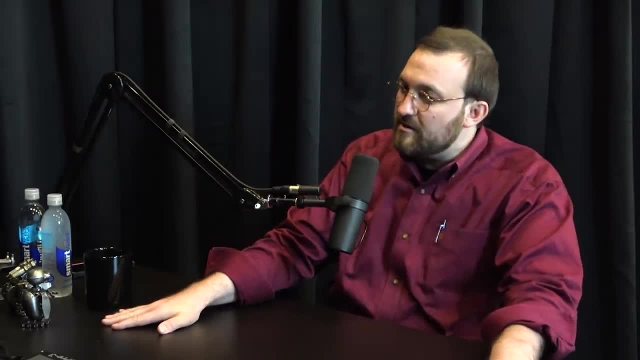 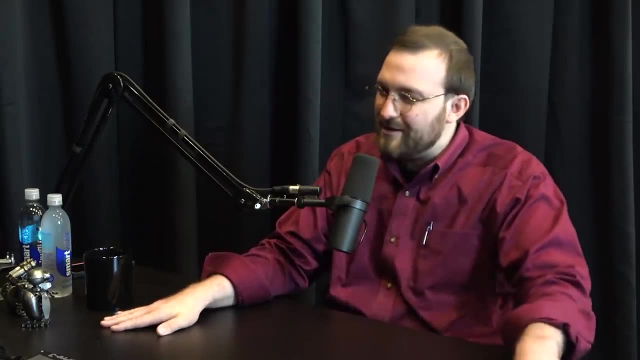 two, And what I mean by that is that you might end up implementing a wrong thing. You might think that what you've built is the paper, but the computer's not going to tell you that, because the paper is written in prose and maybe typed up in LaTeX or something. But 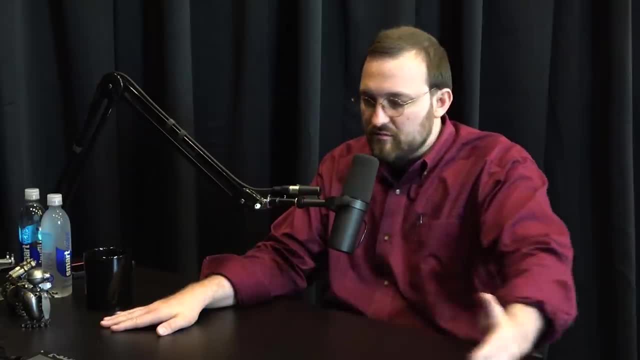 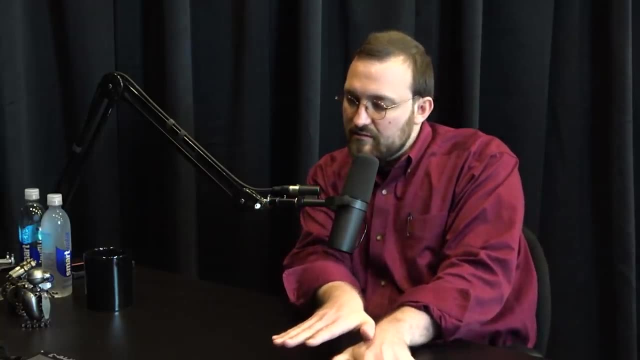 there's no proof chain, evidence chain, that you can show that there's no ambiguity. When you look at a functional language, you're a little closer to math, And so, as a consequence, the translation of the paper is going to be a little bit more complicated, And so you might end up implementing a wrong thing, But there's no proof chain that you can show that the paper is going to be a little bit more complicated, And so you might end up implementing a wrong thing, But there's no proof chain that you can show that the paper is going. 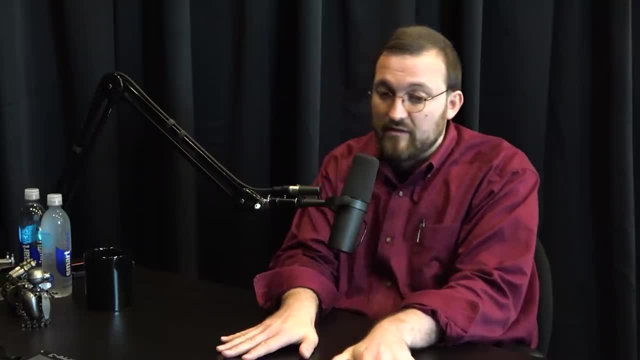 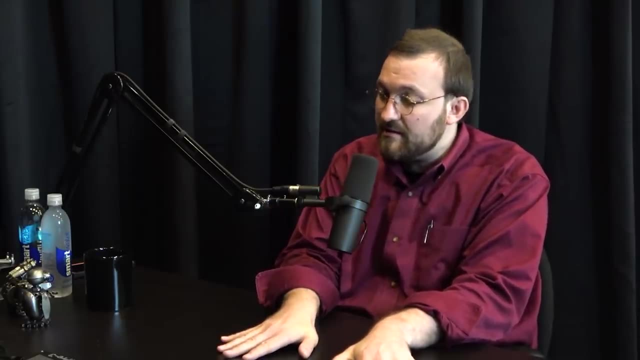 to be a little bit more complicated, And so you might end up implementing a wrong thing. So the downside is these functional languages tend to be a bit more academic and they tend to have not necessarily the best Windows support, and the libraries aren't so good, And also they tend to be a little slower when compared as a whole, on average, to languages like C, for example. So it's really a question of okay, what are you designing for for version one? Are you designing for performance and are you designing for developer accessibility? 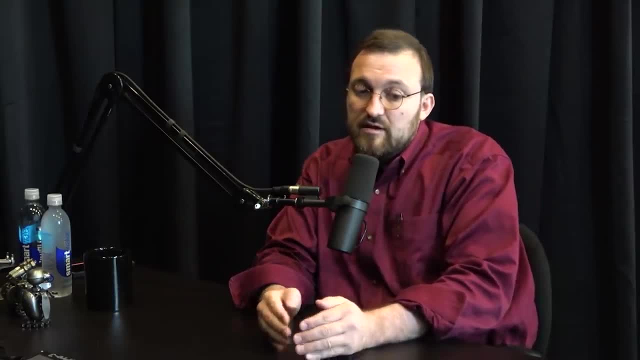 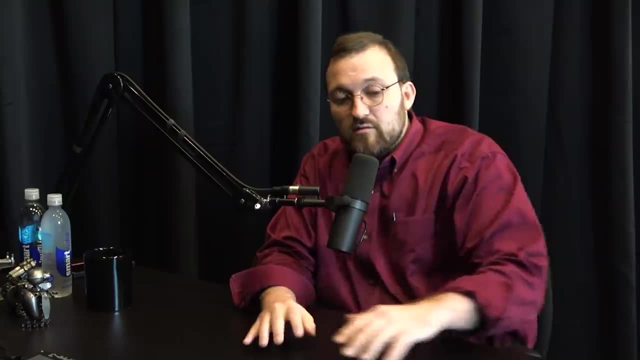 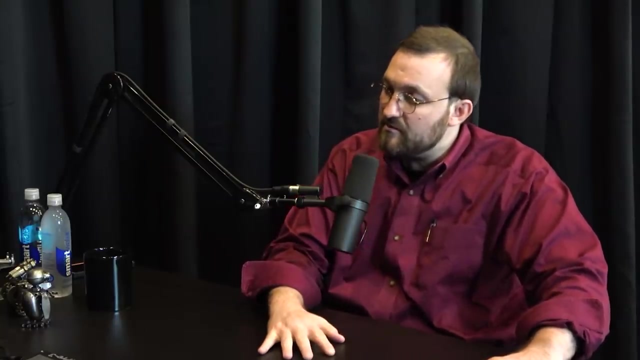 Are you designing for correctness and are you designing for a high fidelity representation of the protocol? Okay, So Haskell was chosen as kind of the version one, because we knew that the kinds of people who think about that are also the kinds of people that would have. 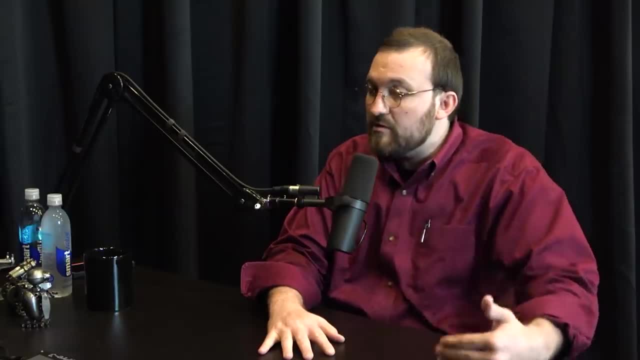 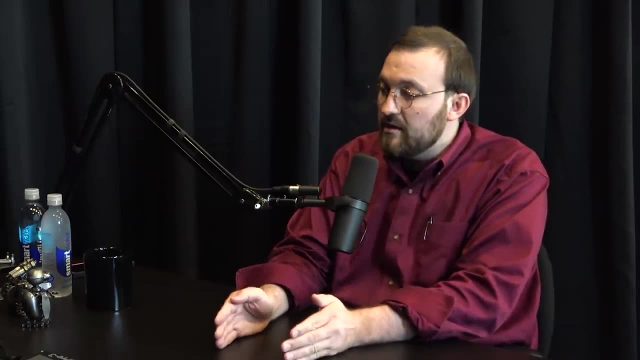 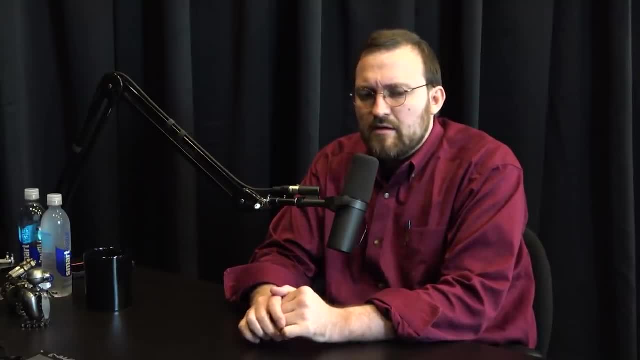 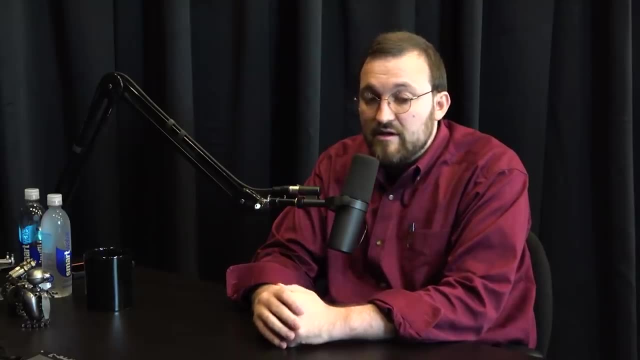 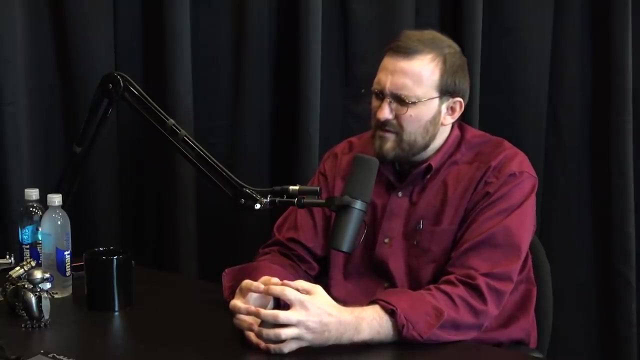 The other side of it is that Haskell code, or functional code, tends to be significantly more concise, And I actually have a real life example of that. So if you take a look at Mantis, we implemented a full Ethereum node. in Scala. It's only about 14,000 or 15,000 lines of code. 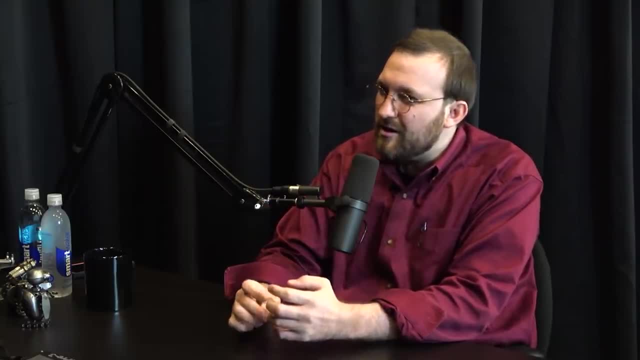 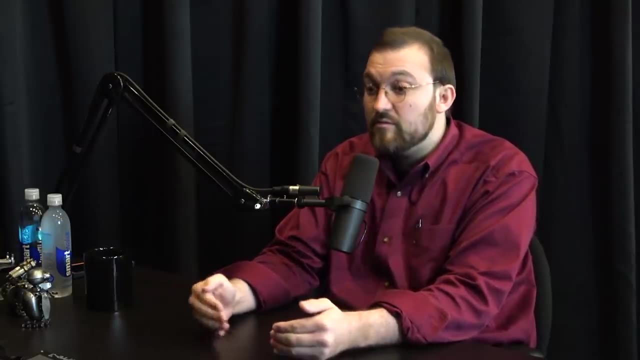 And you compare that with, like C++, Bitcoin, I think that's 120,000, 150,000 lines of code, So it's almost 10 times smaller And so less code, less to read, And you tend to read code significantly more than you would write code. So it's always an advantage for maintenance, understandability, documentation and other sort of things when you have more concise code bases, And also it's a lot easier. It's easier for you to apply stronger tools to a functional code base, like static analysis. 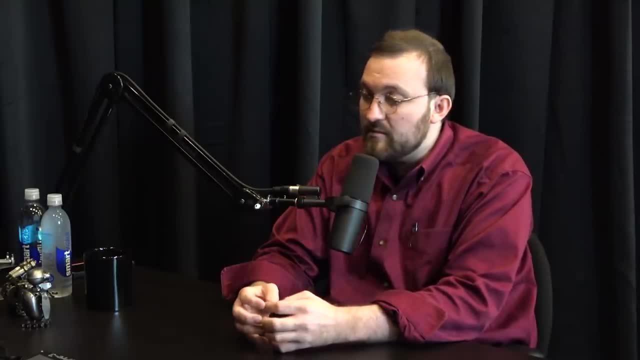 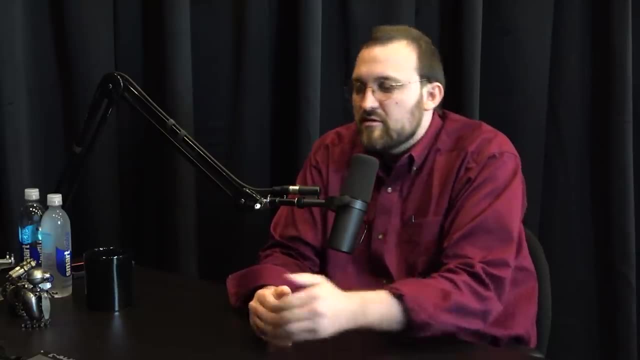 or property-based testing or these types of things than in a imperative code base. But the thing is, it's almost like a religion or language. It's like saying: what's French versus Russian versus English? Everybody has their adherence. They say, oh, they have the best poetry here. 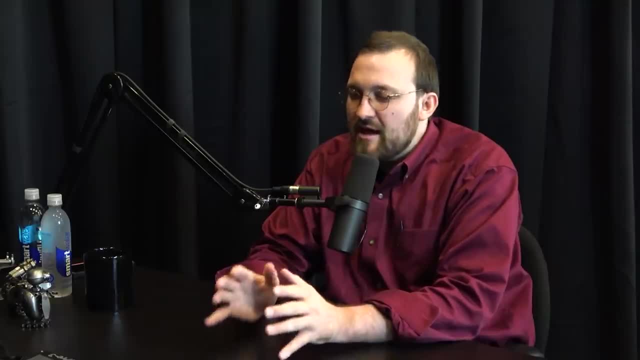 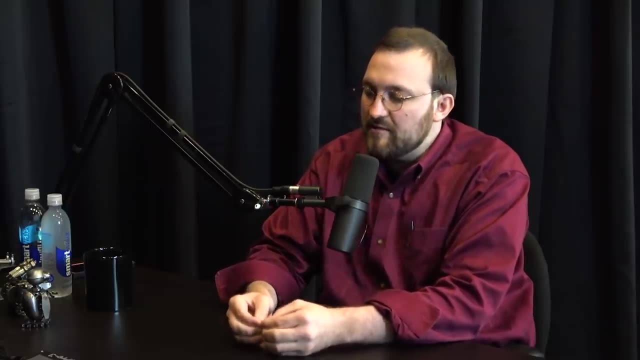 Russian. yeah, There you go, Always Russian. Everybody has their favorite tools and their favorite languages, But it just comes down to what problems are you trying to solve and what problem to be. If you're inventing new protocols based on science, you're going to take the time to. 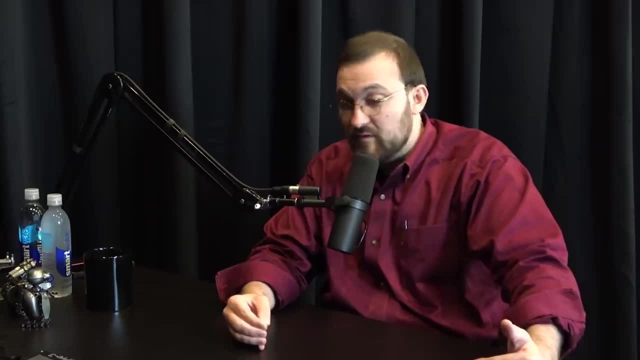 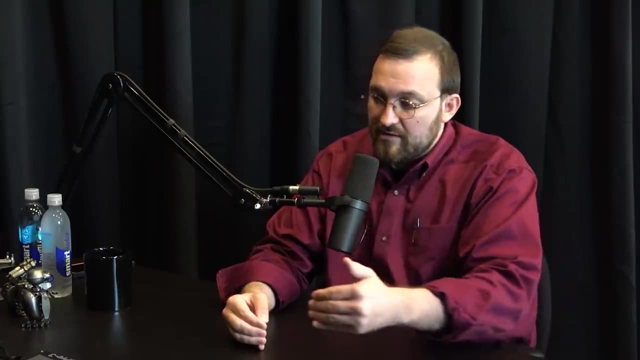 write a paper, go through the peer review process, as you've done personally, and you know how hard it can be to get into a conference and go through that and get your ass kicked. Then you also have to apply the exact same level of care to the engineering side in terms. 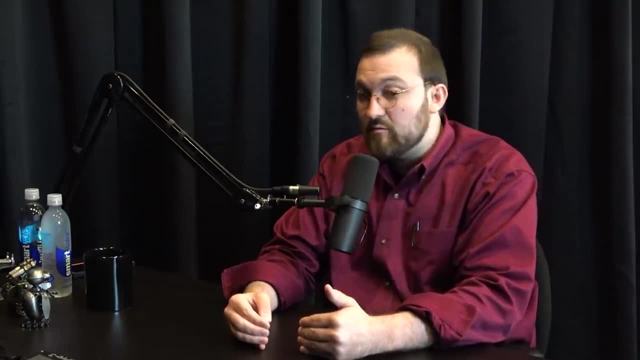 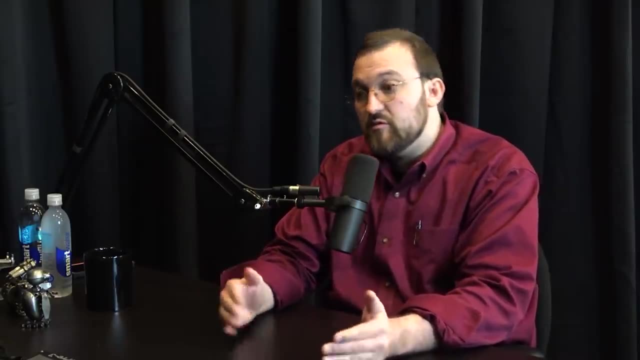 of the implementation of that, or else you will make a mistake, And that mistake will probably be an exploit in the system that destroys the security properties of the system. So we really had no choice but to go to some notion of security, And that's what we're doing. 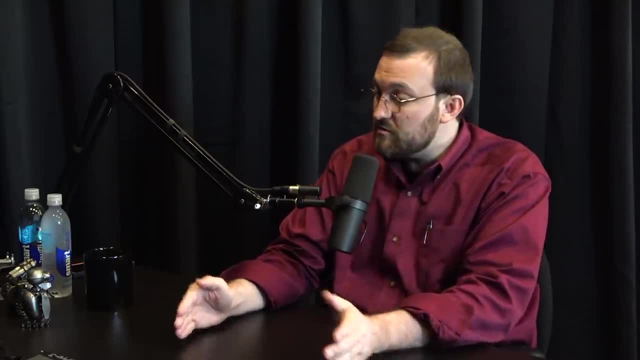 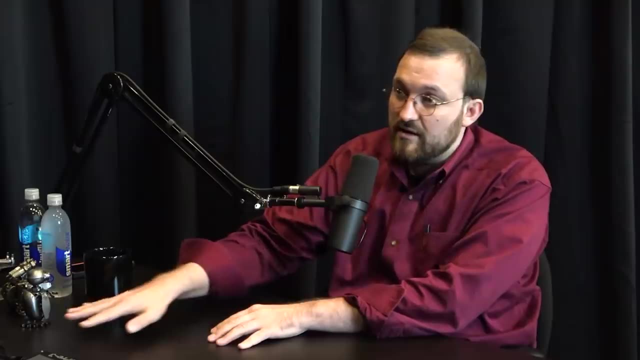 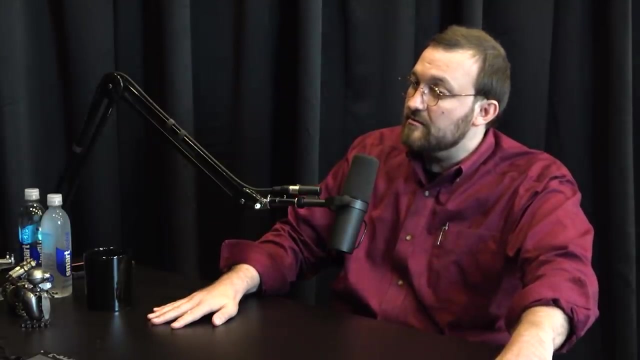 The question was: what's the Goldilocks language? Do you use a hybrid language like Scala and F-sharp or Clojure, where you still have some connection to understandable things like NET or the JVM, Or do you go to an overly academic language like Idris or Agda, or you know Isabel? 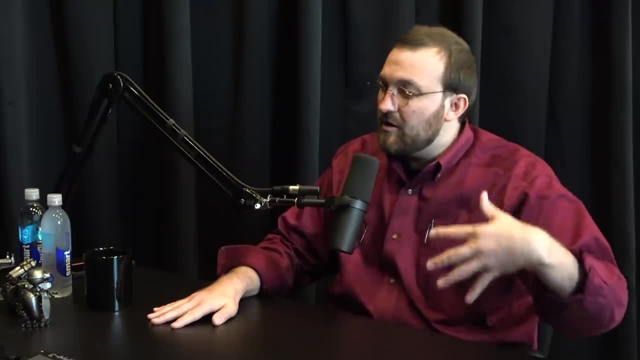 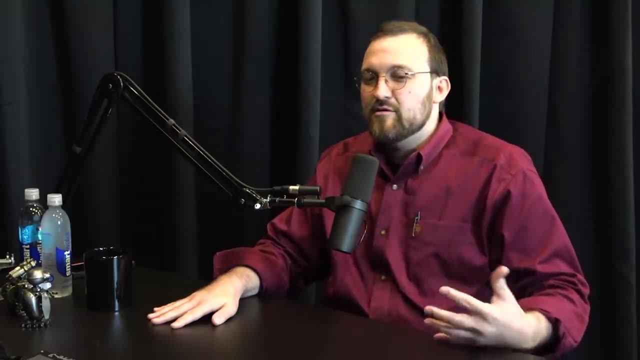 And there you can really dial up the correctness and write all kinds of crazy proofs, But, by the way, it's like the seven people who write your code, they go on vacation a lot. You'll never get anything done. So Haskell, Haskell kind of felt like a nice middle ground between those two where, if we needed to pull, 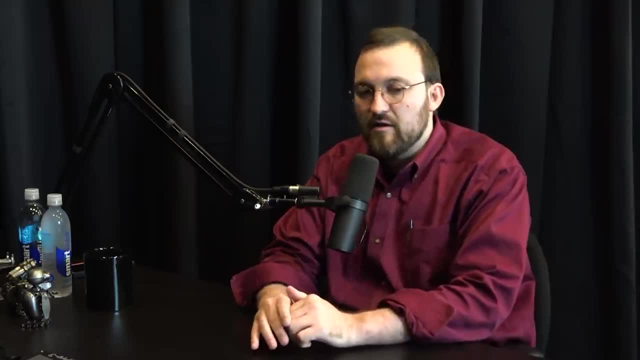 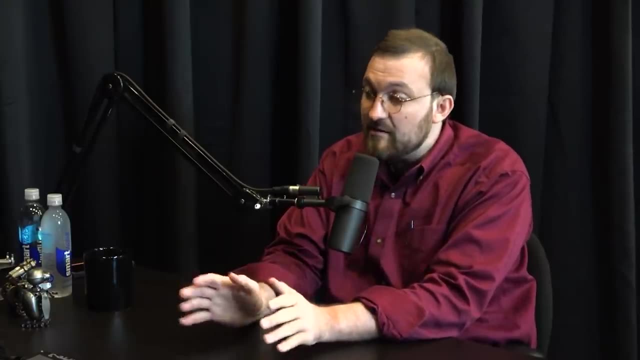 into the left, we could. If you wanted to pull into the right, you could as well. That said, it's really amazing to see what the hybrid languages have done. If I was a new student in computer science and I said: you know, learn any language to. 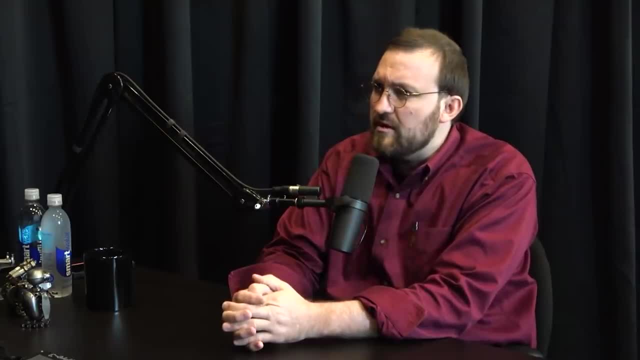 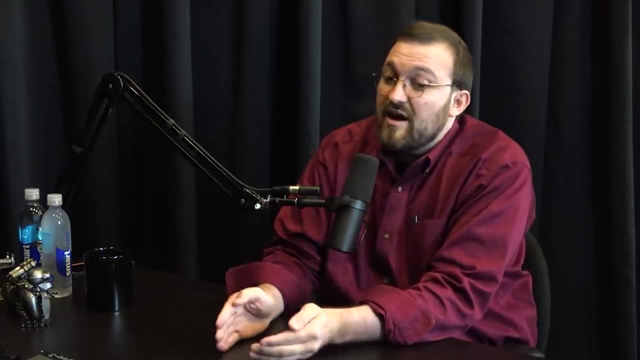 grow your career from. Scala 3 is probably the language to go with. Yeah, it's great because it's like you want it to be like Java. It's Java And it looks kind of like a Java program. You want it to be like Python and scripted and you reuse a REPL. 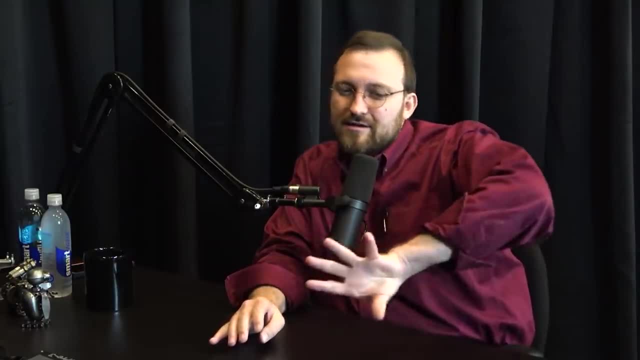 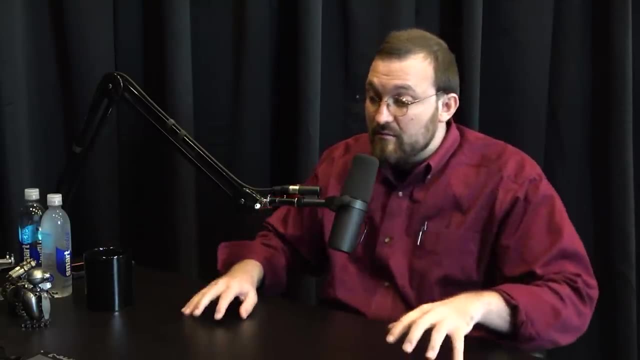 You can do that. You want to go hardcore, dot. you know dependent object types and do like weird proofs and stuff and the functional. you do all that. You have access to all of these things And Martin Adersky is a brilliant guy. 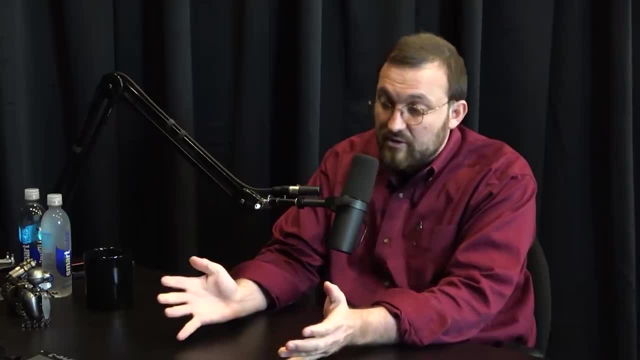 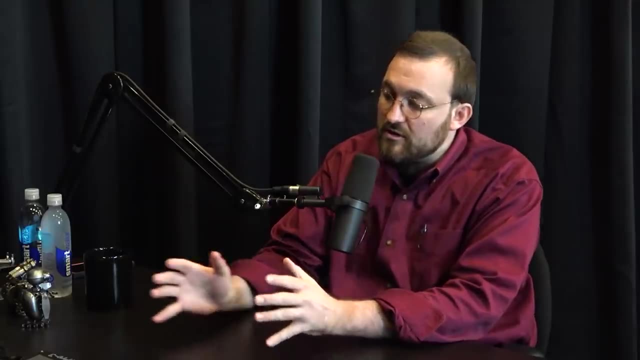 He's done some phenomenal work, basically because he was one of the guys who created the JVM and he's worked on compilers for over 20 years. He did a lot of really hardcore work in trying to build a concise, nice, modern language. 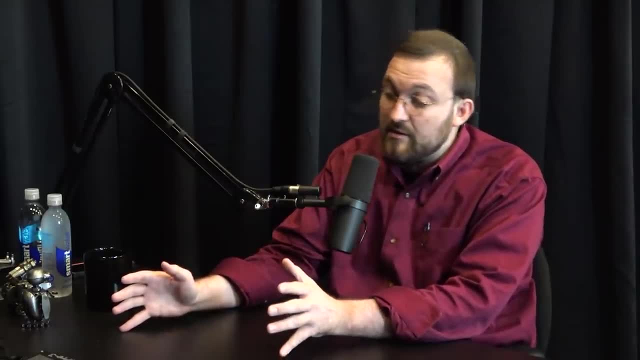 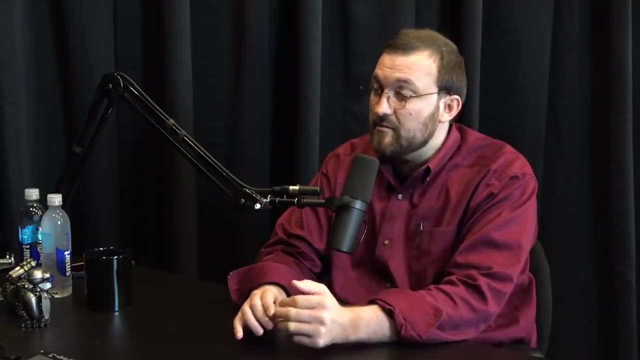 that does a little bit of everything And it's got great applications in data science And it's also heavily used in modern companies like Netflix uses Scala for all of their microservice architecture. Yeah, So there's. that's a great language and it's easy to pick up and it's easy to hire people. 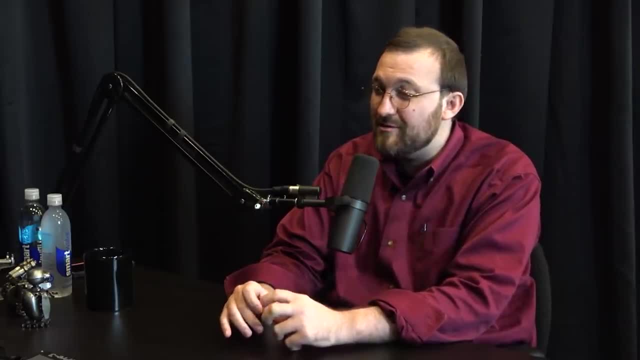 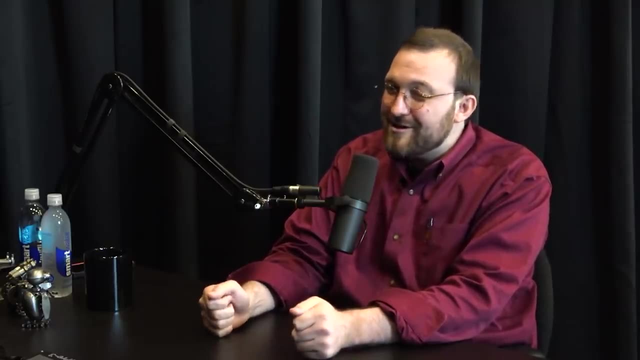 into it. You just find these Eastern European guys who were Java programmers for 10 years- 15 years- and they got tired of making $20 an hour, So they picked up Scala. so they can make $35 an hour and they're really good at it. you. 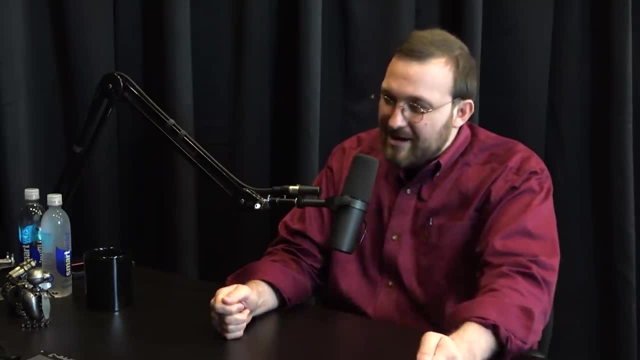 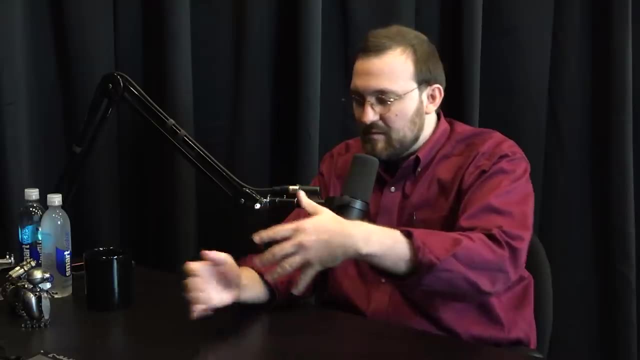 know- And that's a great gateway drug because you know you have like QuickCheck and Haskell, you have ScalaCheck and Scala. you know you can also build, do a lot of things. You can do model checking. You can also go and use a TLA spec and make it work with Scala, and so forth. 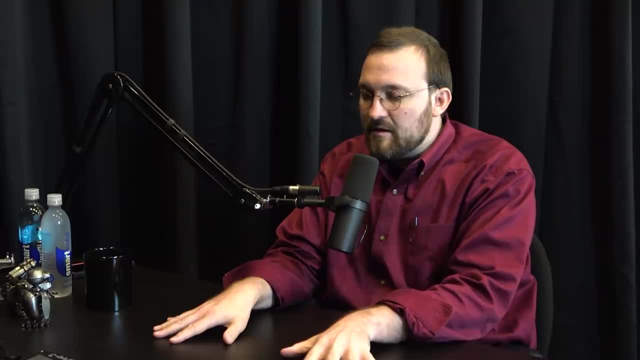 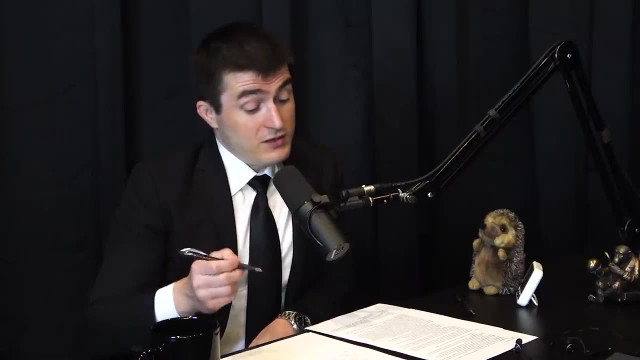 So it's. it gets you a little bit of everything and you know you can then move around that entire design space in a beautiful way. So the recommendation is maybe, if you want to go vanilla, you go Python and JavaScript When you're getting started.